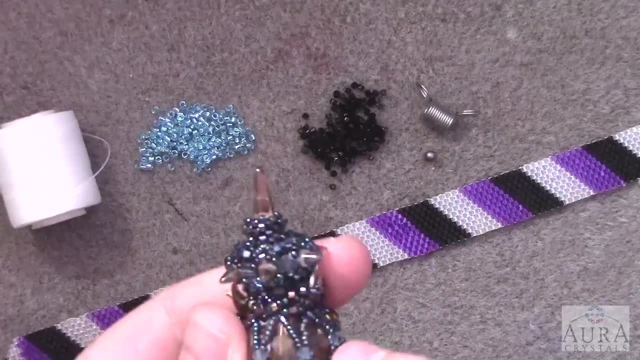 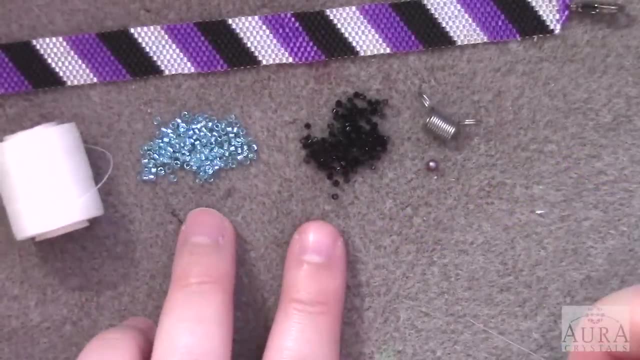 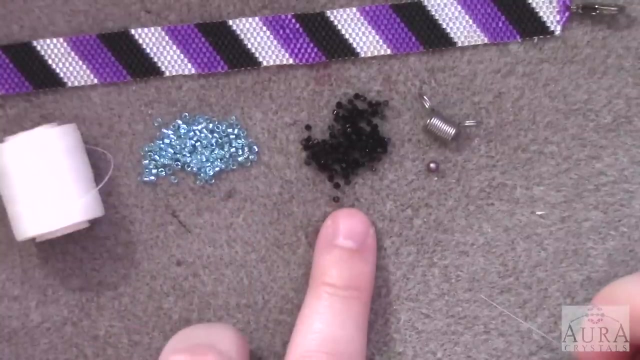 it in a wide variety of jewelry applications, including creating 3D structures and pieces such as this. For this project, you will need two contrasting colors of Delica beads. I'm using Silver Line Turquoise- number 149, and Opaque Black- number 10.. These are both in. 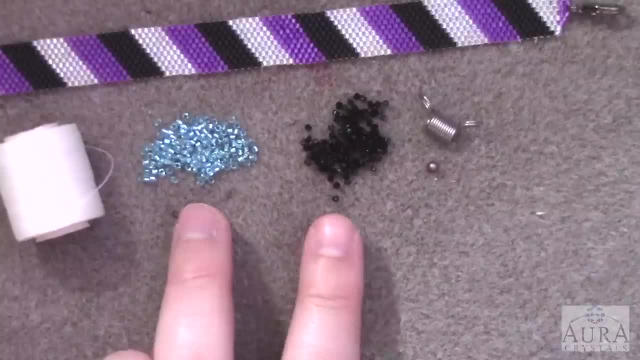 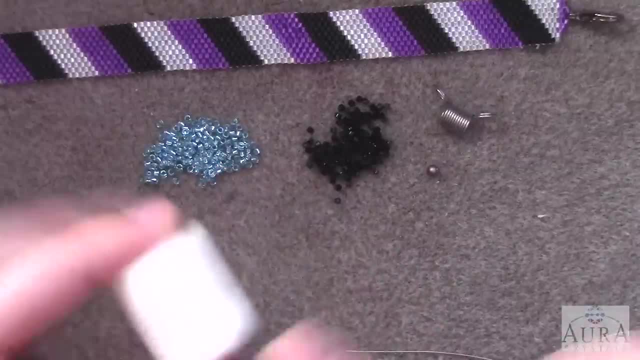 to work with, Since you won't have to worry about uneven beads. you can just use whichever thread. I'm using a D-weight Nymo and I'm using a size 12 needle, but you can also use a size 10. 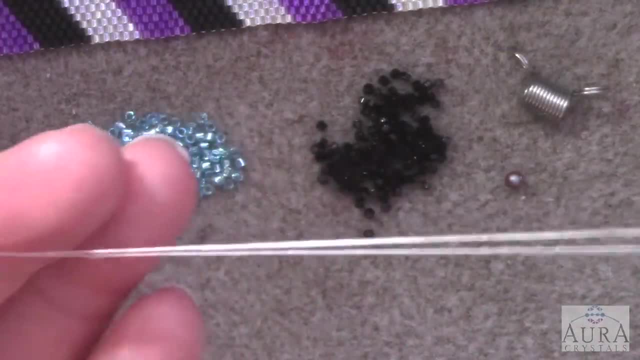 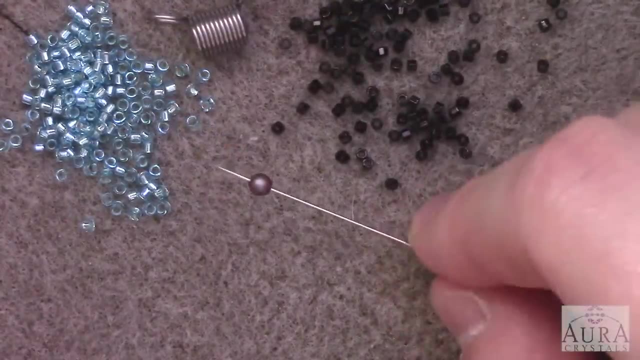 if you'd like Start off by threading on about a yard's worth of thread. You can always add more later. So the first thing we need to do is to thread on our stop bead so that we can keep our beads on our thread while we're working with it. So I'm going to pass that down, leaving about a 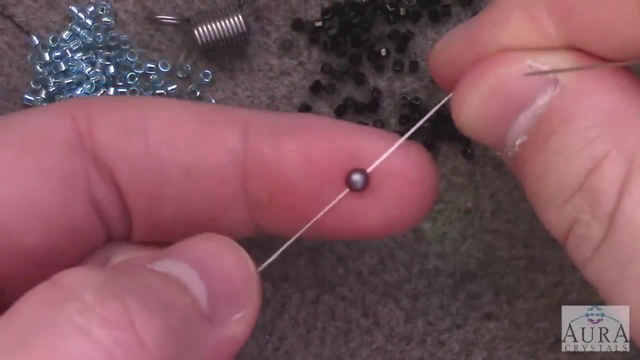 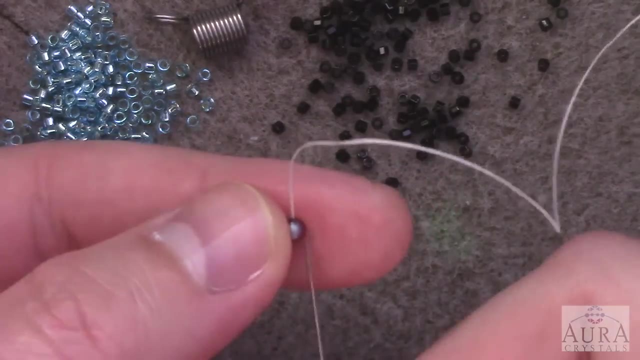 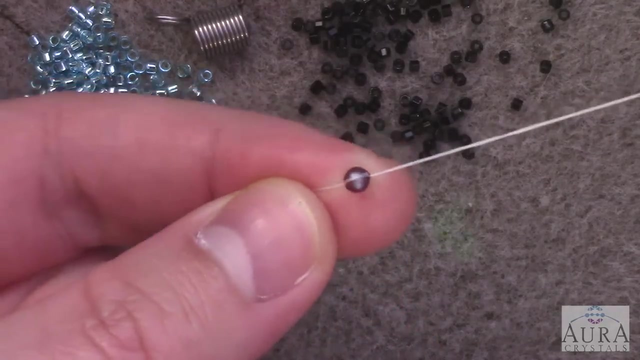 six inch tail, so that I have enough room to tie off my ends properly. Now all I'm going to do to secure it in place is to pass back through the bead once more so that the thread is caught in there and it wraps around the bead once. If you have a spring bead stopper, all you do is open it. 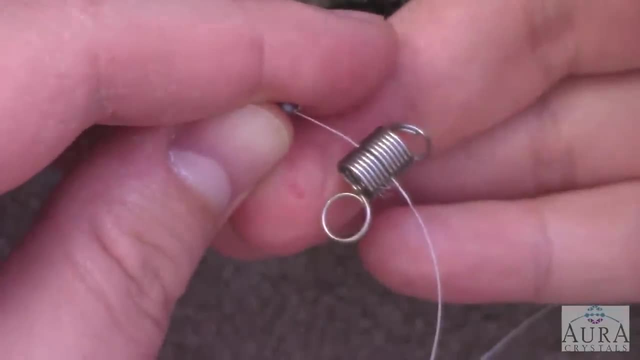 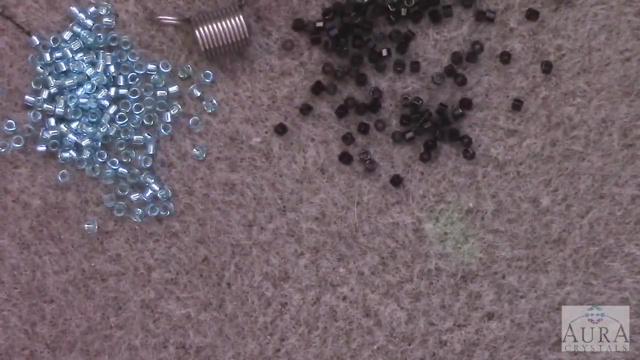 up and slide your thread through one of the gaps and close it shut. Now even Count Peyote gets its name because there's an even number of beads per row. So in this example I'm going to put four beads per row. Now, the first row is much different than 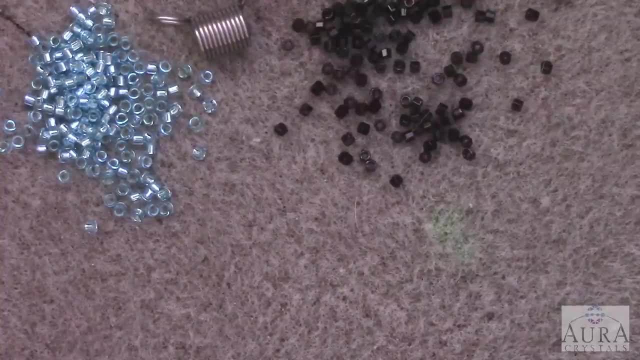 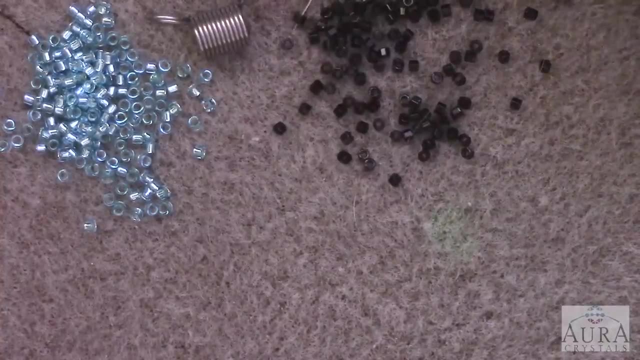 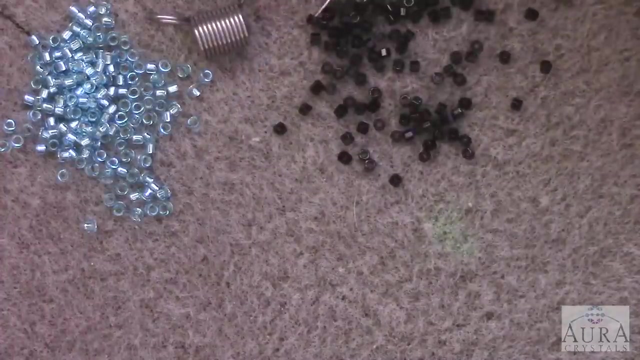 the rest of the rows that we're going to work with, and usually with a lot of different beading stitches. the first row is a little bit more difficult than the rest of it, So I'm going to start off by threading on an alternating set of beads of blue and black until I have four of each. 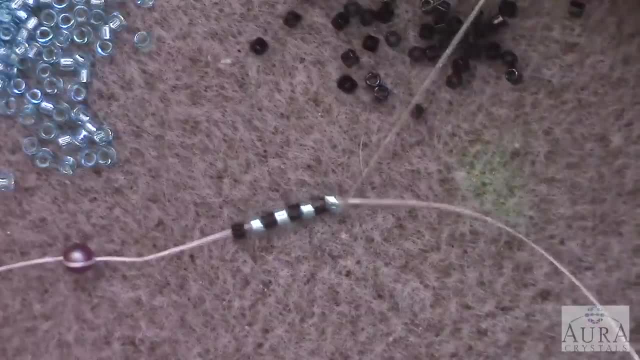 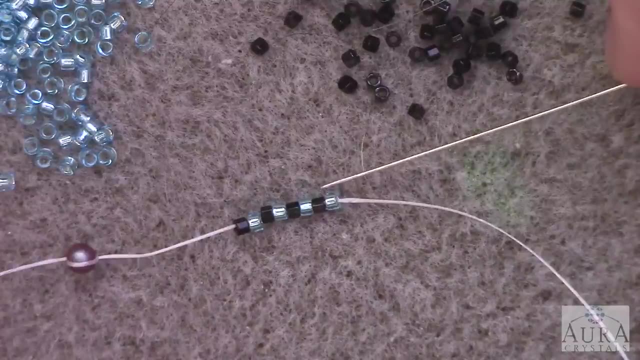 beads, And this is what our starting row is going to look like. In this example, all of our odd number rows are going to be the blue and all of our even numbers are going to be black. So, since we have two rows working with at the same time, our next 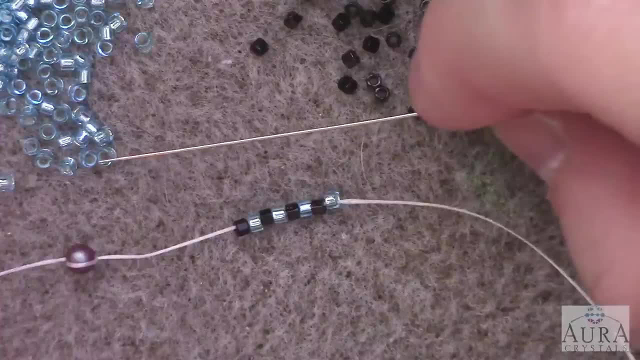 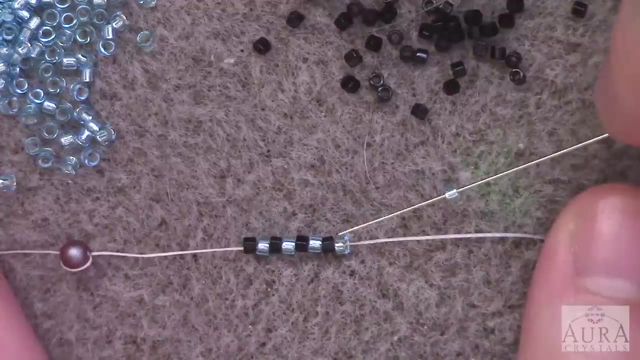 row is going to be row number three, which is odd, so it's going to be blue. So, in order to add on the next row, I'm going to take one blue bead. I'm going to skip over the last blue. I've added. 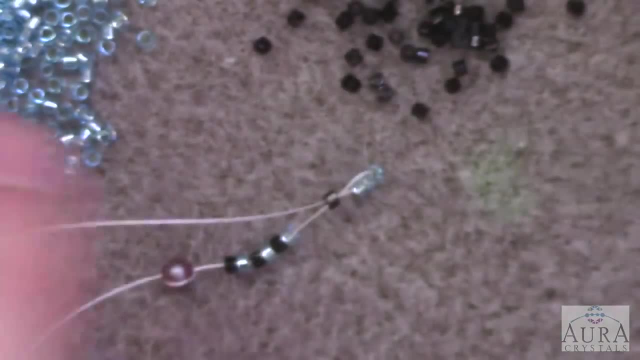 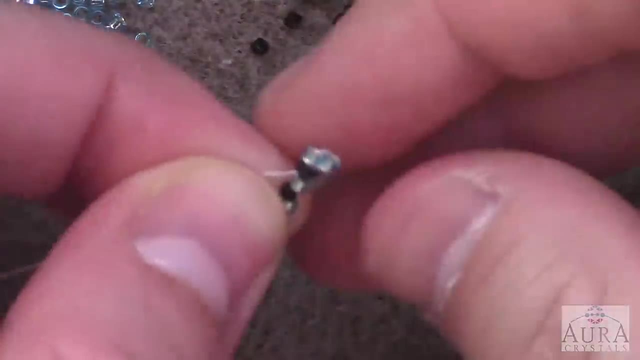 and pass through the black, And when I pull that tight, I've captured my two blue beads here. What I want to do is pull it tight and flip it over so that the two beads sit on top of each other. It's very important to keep your 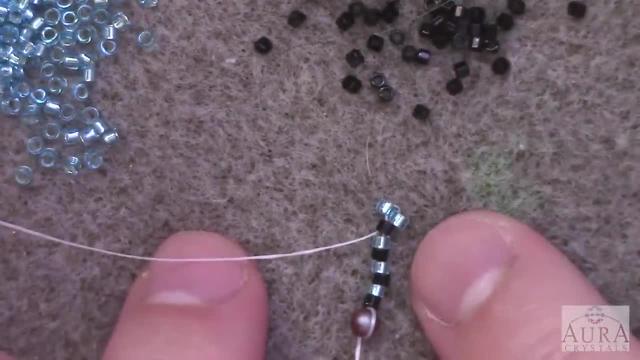 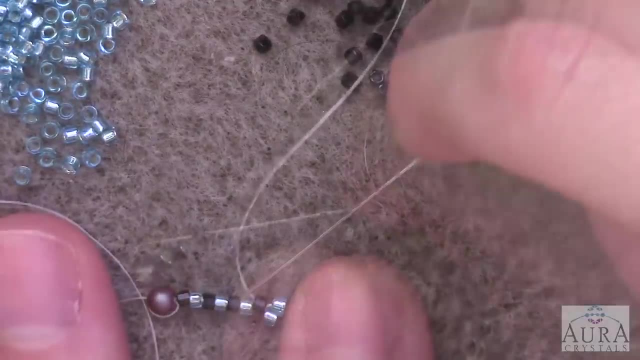 thread tension fairly tight to maintain this structure. Now for the next stitch. I'm going to repeat the same thing. I'm going to add one blue bead, skip over the next blue bead, then pass through the next black bead And when I pull that tight, the next bead. 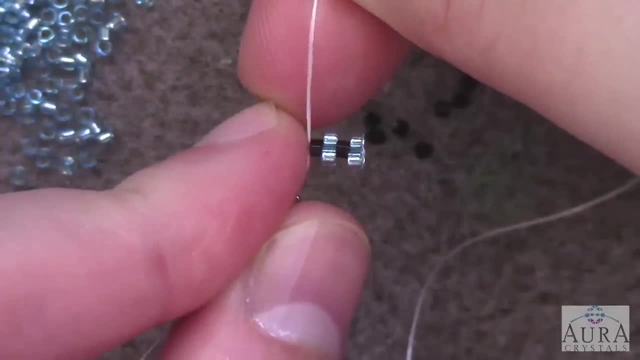 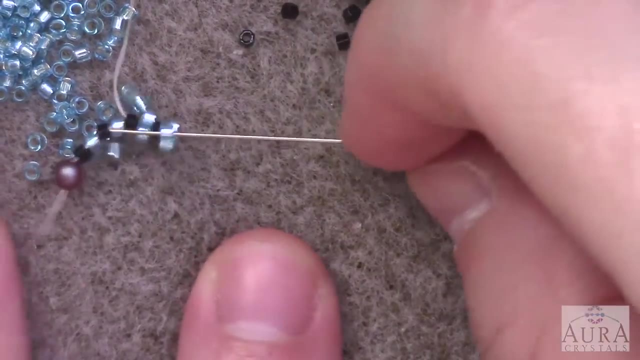 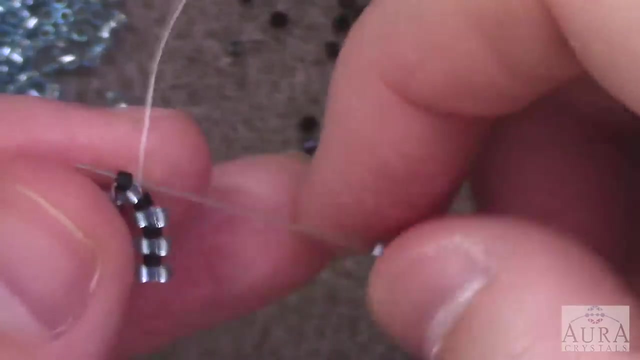 is sitting right on top, wedged between the gap between the two black beads. And I continue on this way: add on one more bead and pass through just the next black bead, Add on one more blue bead and then pass through our final black bead. And this is what our first three rows look like. 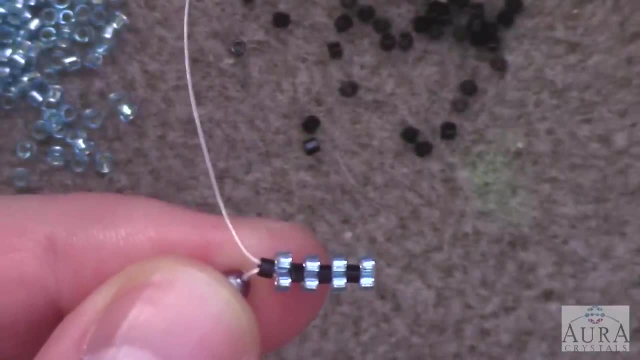 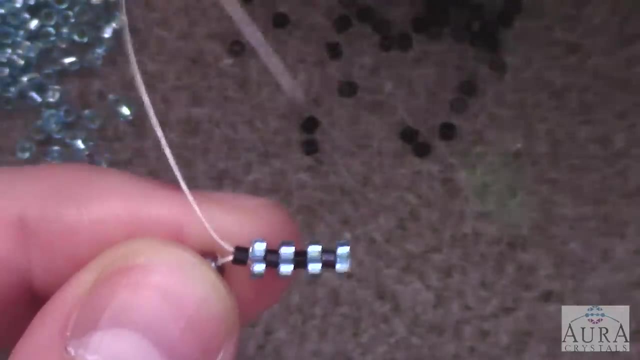 Now we're on row number four, which is an even row, So we're going to be working with black beads this time. So, Coming out of the very last black bead, I'm going to add one, then pass my needle through the next blue bead, skipping over the black. 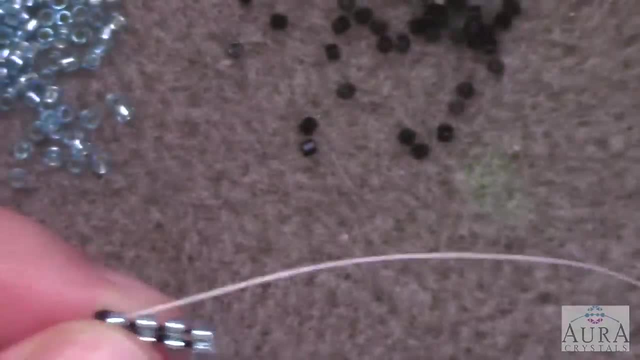 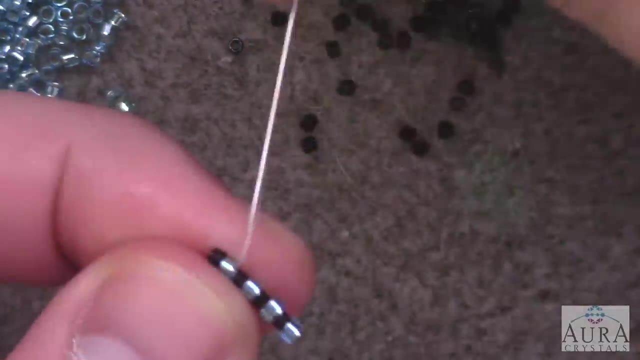 We have two black beads on top of each other. I'm just going to continue in the same way in order to finish this row. So I've added one black bead. I'm going to skip over the next black bead and pass through the next blue. 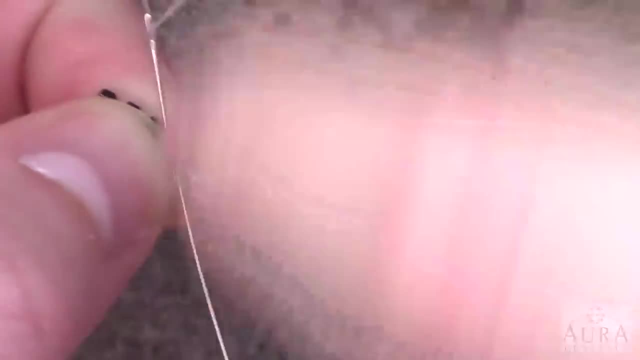 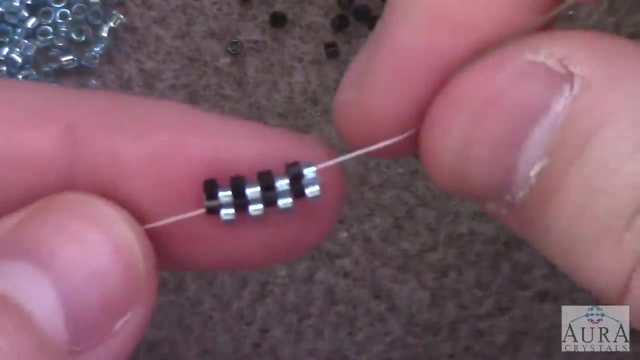 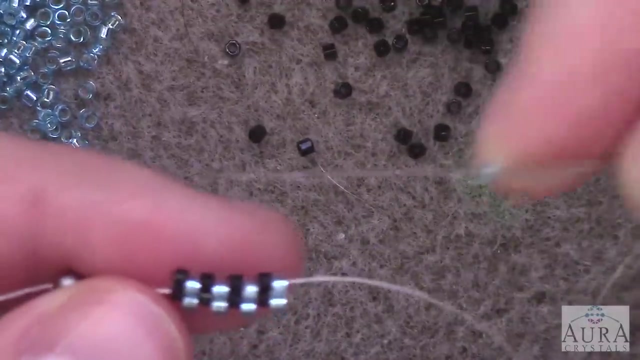 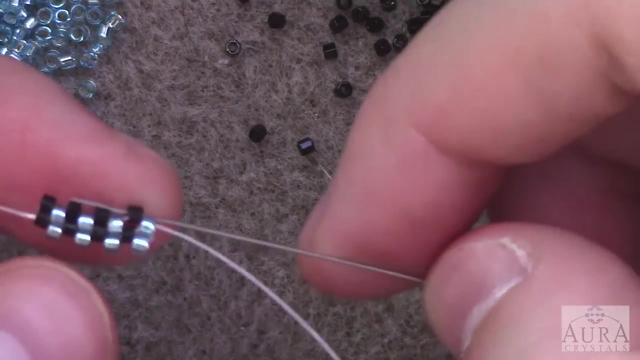 Add one black, pass through the next blue, Add one black and pass through our final blue. And now I have completed row 4, and I'm back on the blue side, starting row 5, so we switch to blue. Coming out of the last blue bead, I add one more blue bead, skip over it and pass through. 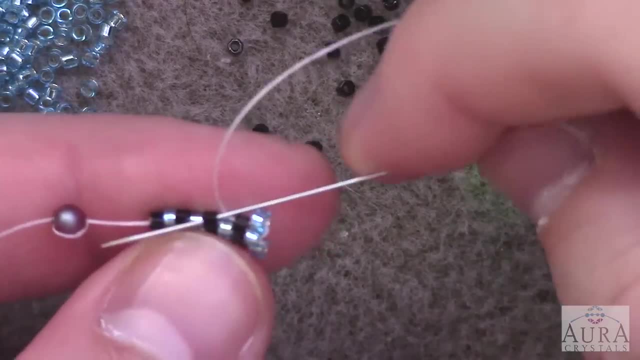 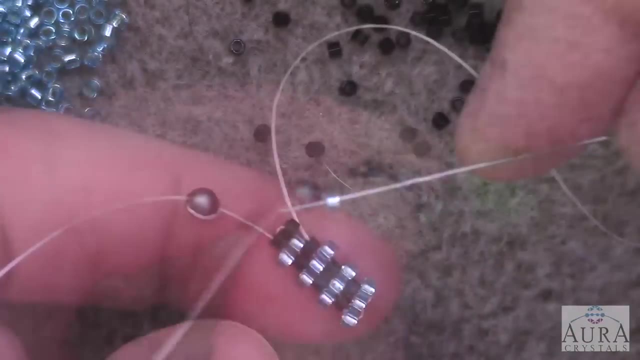 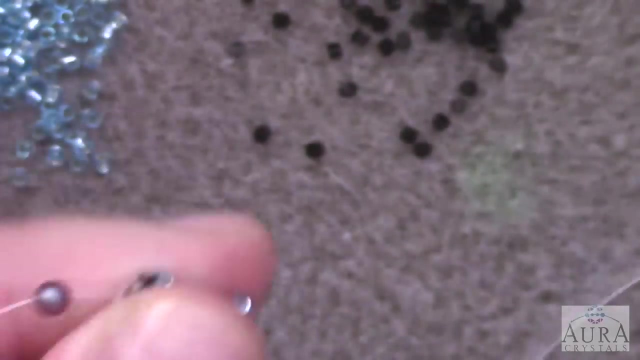 the black Once more. add a bead. skip a bead. Go through the black. Add one bead. skip a bead. go through the black. Add one bead, skip a bead. go through the last black, Like so. Now I'm ready to turn around, starting with the black, going through all the blue beads. 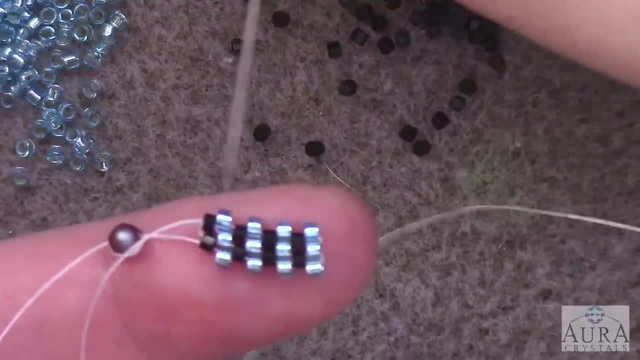 on this row, And that's basically how you do it. You go one direction, turn around, go the other direction. turn around, go the other direction. Now, If you're not too comfortable with the blue beads, you can do this. 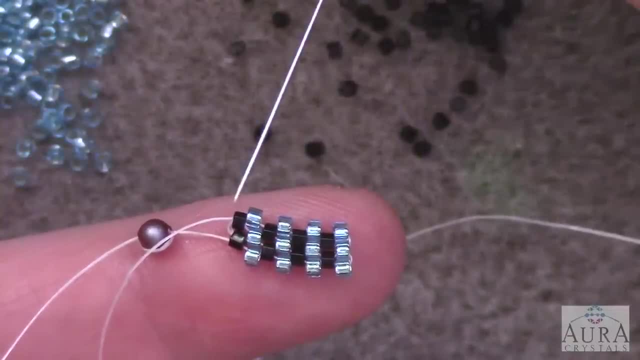 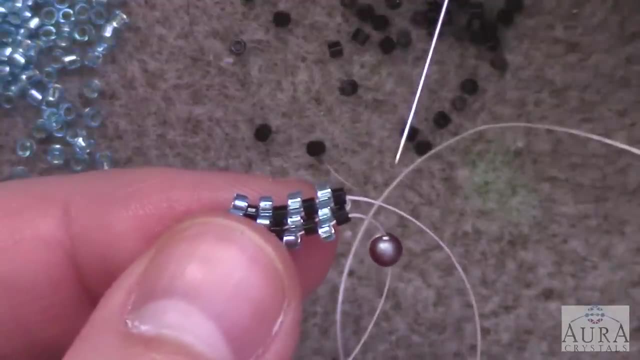 If you're not too comfortable with going back and forth, yet you can always, since I'm starting on this side, if I just flip it over, I'm starting on my right side again, So then I can just add a black bead, go in the same direction. 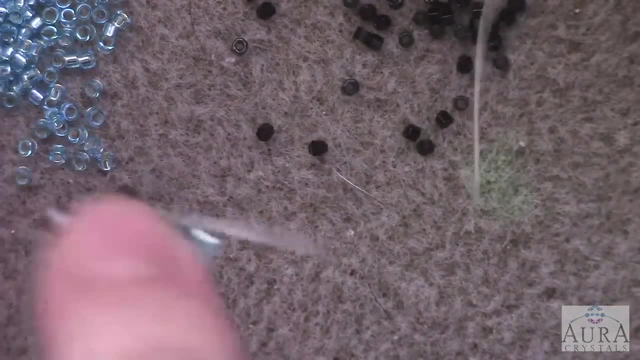 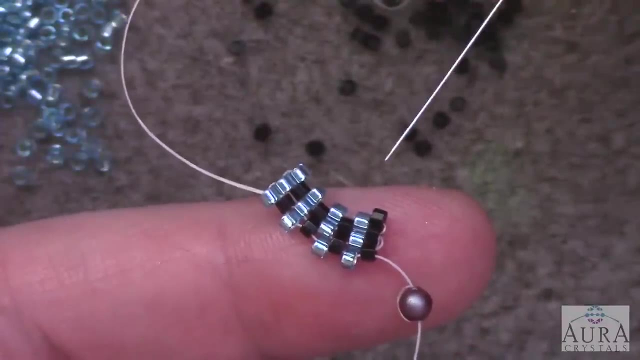 Like. so When I get to the end- blue bead- I can just flip it over and I'm back on the right side. So keep going at this back and forth until you have about an inch of length, and then I can show you how to add threads and end your old ones. 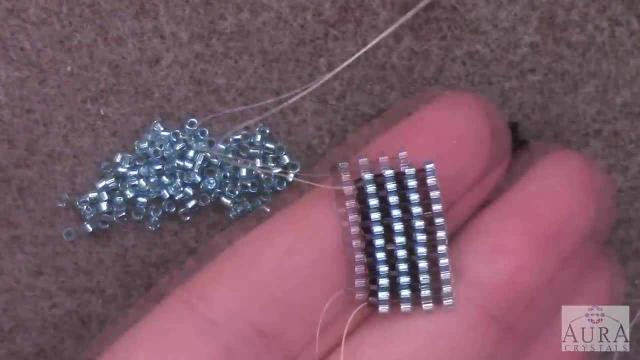 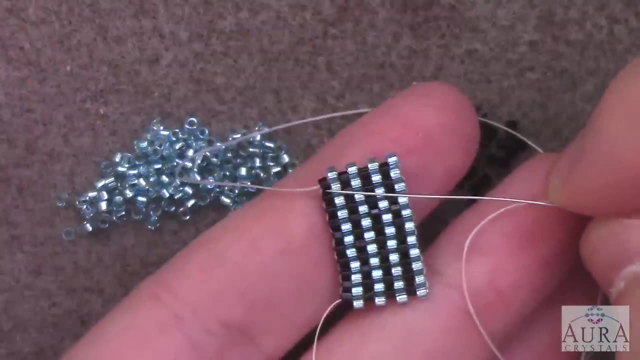 So once you feel that you're running out of thread- which is about three inches or whatever- you are feeling uncomfortable working with it- you want to make sure that you finish off a row. This just helps you keep track of where you were in place so that you don't have to start. 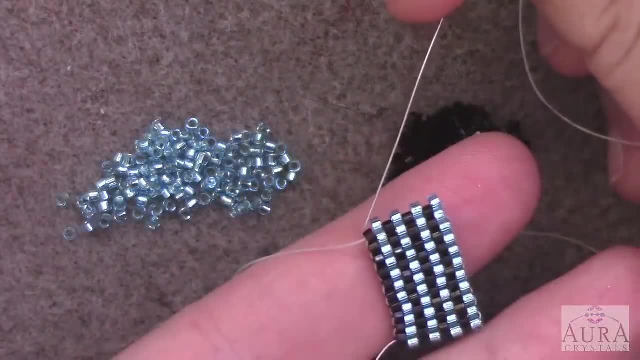 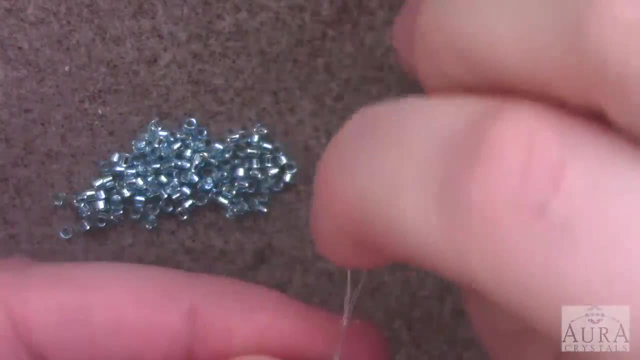 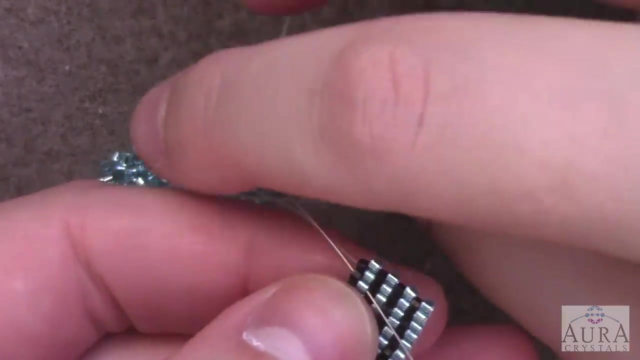 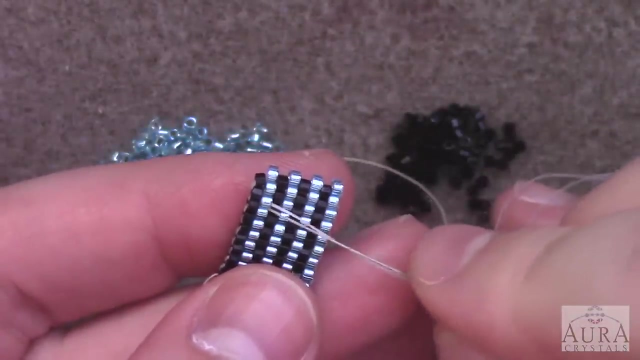 off in the middle of a row. Keep in mind that we've ended up coming out of the last black bead on this row. All I'm going to do is pass downward through the piece, So I'm just going to keep starting off. I'm going through the next black underneath and we're going to kind of do a zigzag motion. 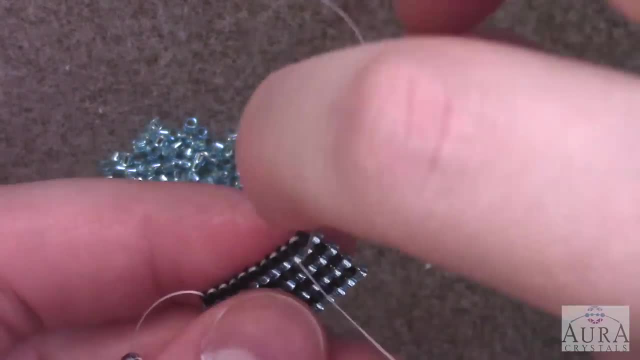 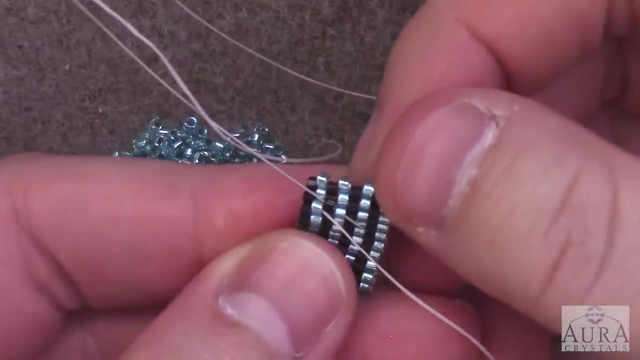 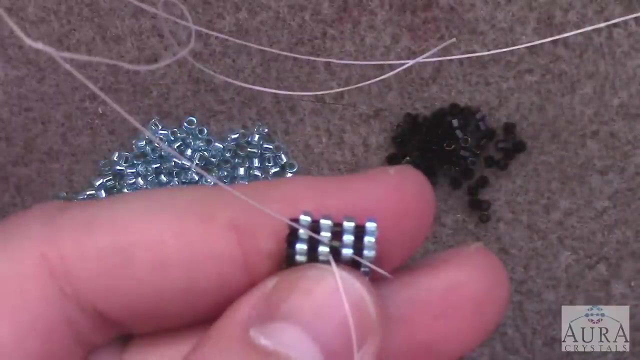 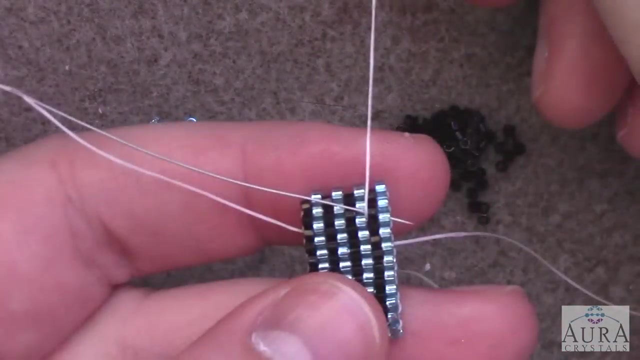 going across the whole piece. So from here I'm going to go up one and down one. I'm going to take my needle and just pass it through the next black above and the blue below and keep doing that, going through the next black and the next blue and finally, until we're at the end of the 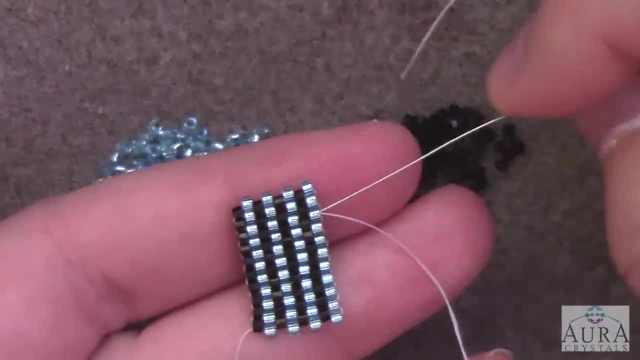 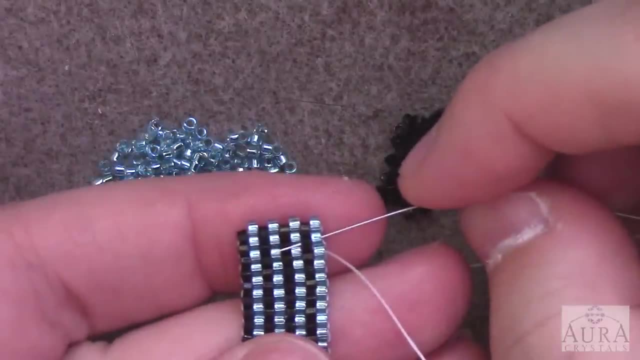 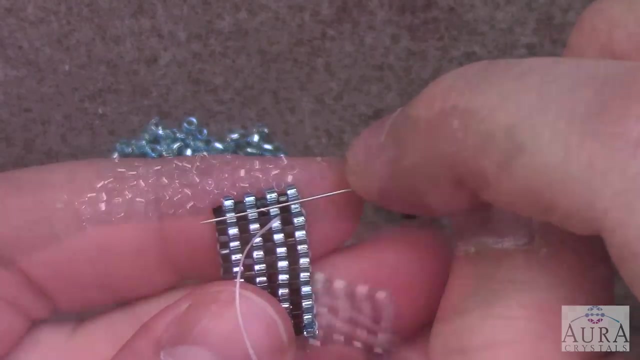 piece. This by itself is reasonably secure, but if you're feeling uncomfortable you can go back through and pass in the opposite direction. So now I'm just going to go up and pick up the next blue and black and keep going down until I'm back out at the black again, like so. 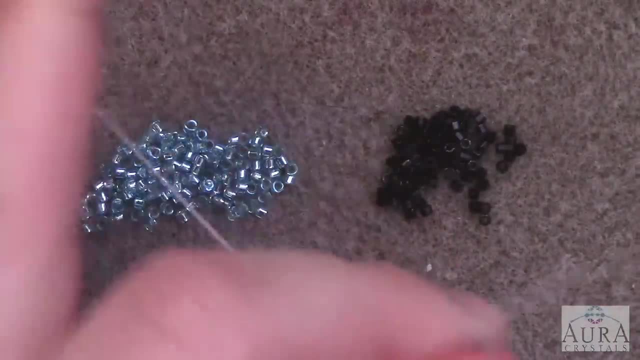 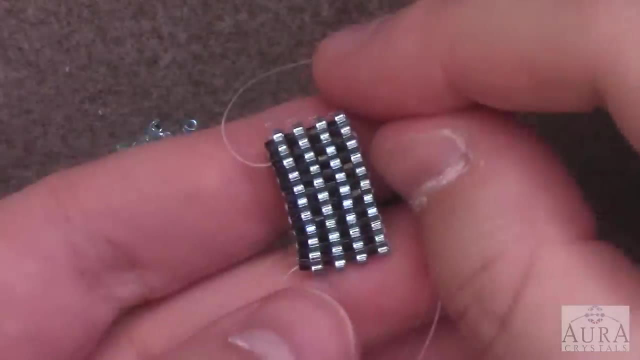 Now be careful when you're doing this with smaller beads. You only have a certain number of passes and you don't want to fill the beads with too much thread. otherwise you'll have a hard time adding in your thread and you take the 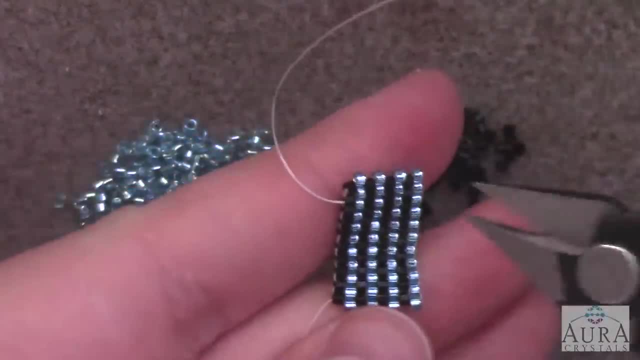 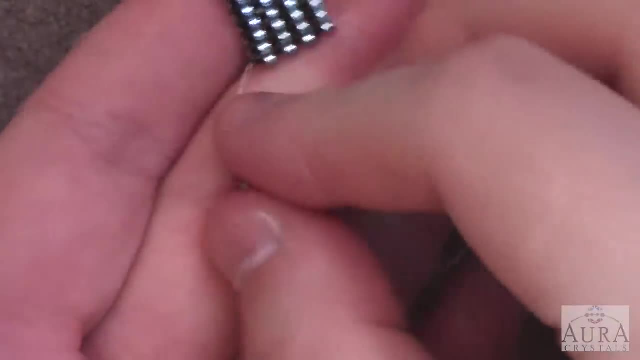 risk that you could snap a bead in the middle of your piece. Once you feel like everything is nice and secure, you can go ahead and clip your excess thread. You can also then remove your stop bead just by pulling it off and end the thread here. 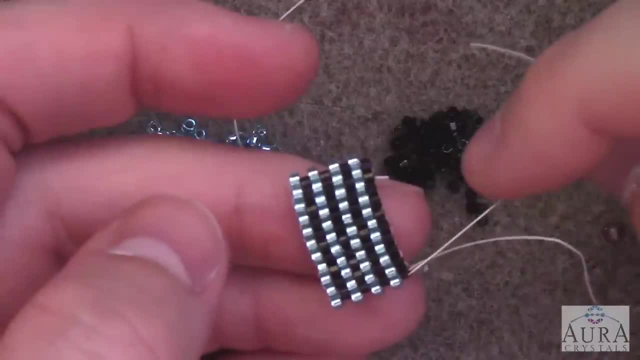 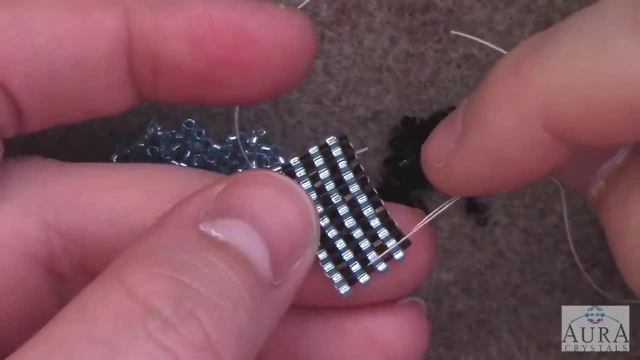 the same way that you did up here. So once you thread your needle, you'll just pass up through the black That is right on top, and keep going through a blue, a black, a blue, a black until you're all the way at the end. 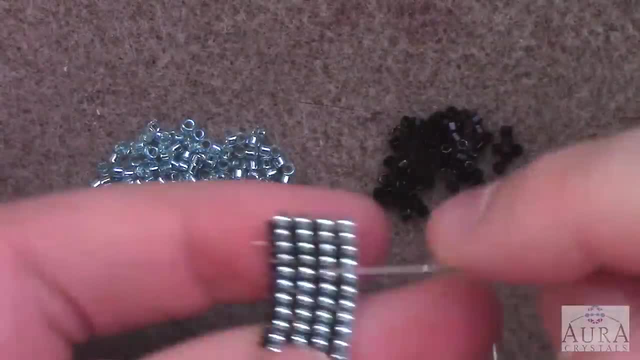 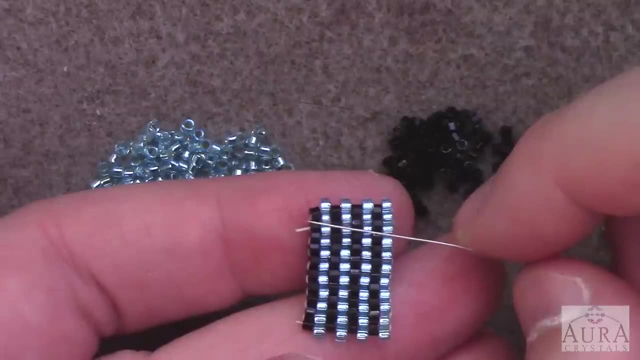 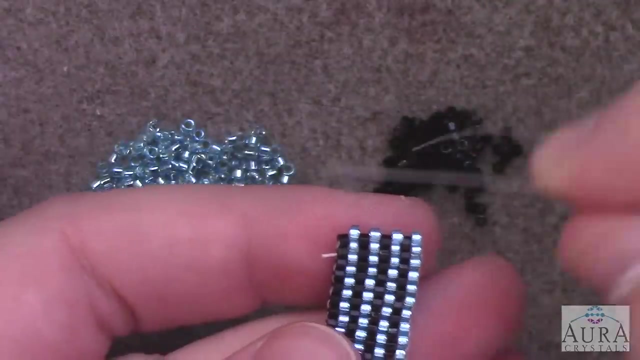 So next you'll need to add on your thread. What you can also do when you're ending your previous thread is maneuver it through the bead that you ended up with when you started off, when you finished your last row, so that you can tell where you need to end up. 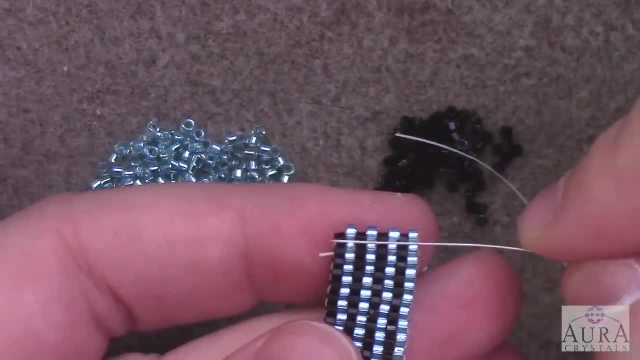 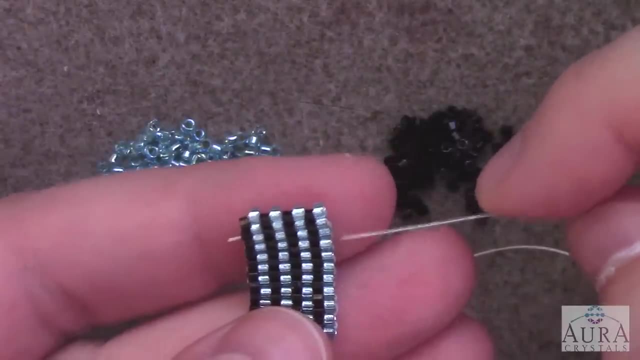 But since I ended my thread here, I know that I need to end my bead up here, So I'm going to start off on the opposite end and basically do the same exact thing. I'm going to start a little lower and I'm going to start my thread up about four rows. 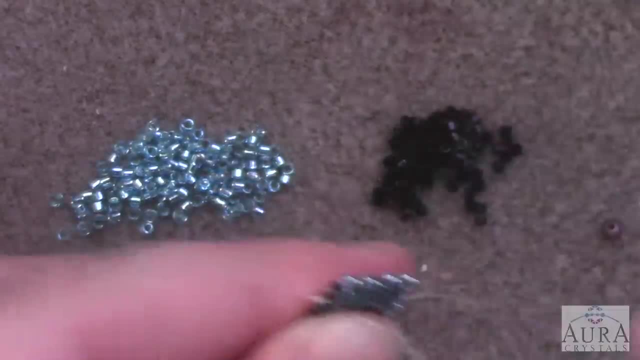 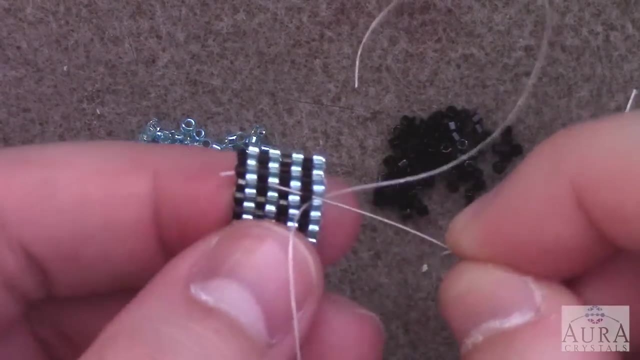 down and I'm going to work my way up. So from here I'm just going to move through the black bead above. I'm going to leave a little bit of a tail so that in case I pull too tight, I don't.